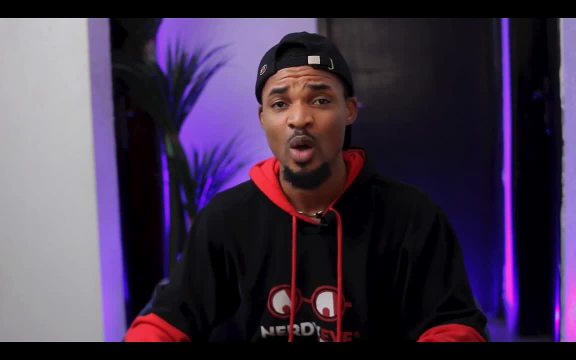 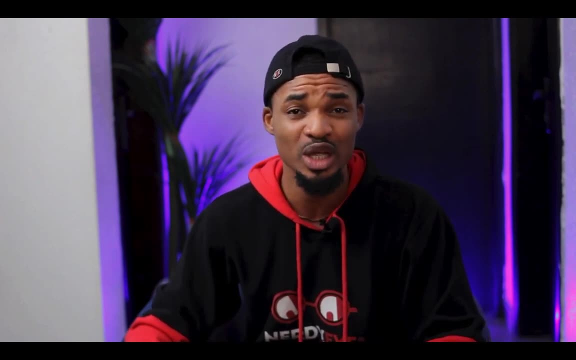 with Nerdy Eye, you have access to all of those things and even more. When you enroll for our platform, you have access to a one-on-one mentor. you'll be able to schedule a clarity call with your instructor at will. you will also join a support group where you can ask questions at any. 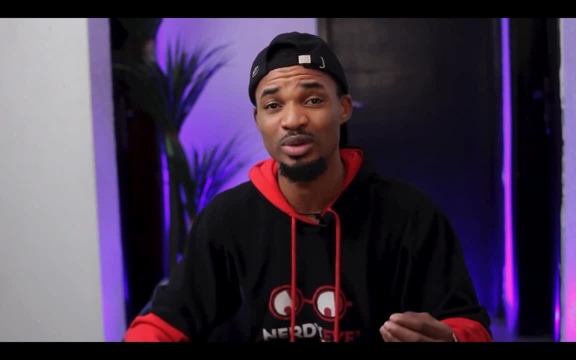 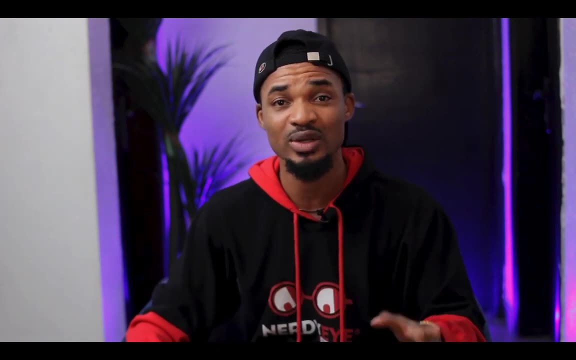 point in time, you will also be part of a weekly live class where you'll be learning and growing with other people. and guess what? You will also be paired with an accountability partner, somebody that you guys can learn and grow with and also build rapport as you advance in your career. And 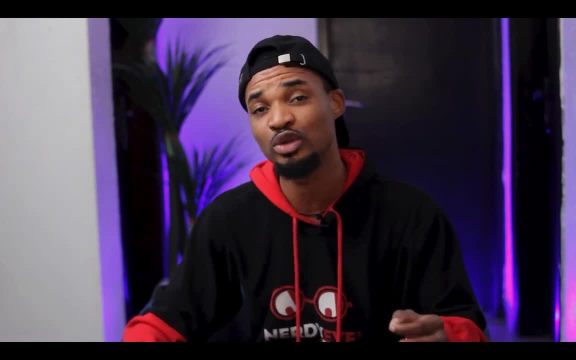 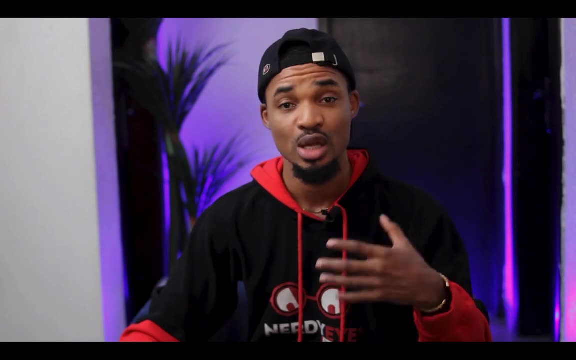 at the end of the day, you'll be able to learn and grow with somebody that you guys can learn and grow with, And at the end of the career roadmap, you also get personalized portfolio review and job support. Don't forget to go on our platform and turn on your subscription. It's just a monthly. 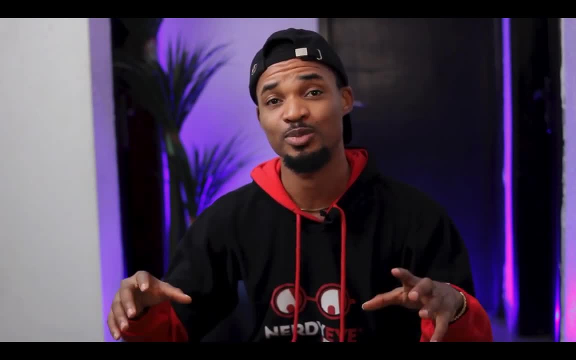 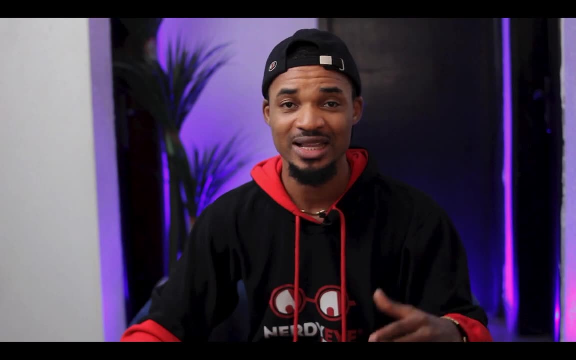 token. That being said, don't forget to also subscribe on this particular YouTube channel, so you'll be notified when we upload subsequent lessons. right? So, without wasting much of our time, let's get into this particular video. Welcome back In this particular video. 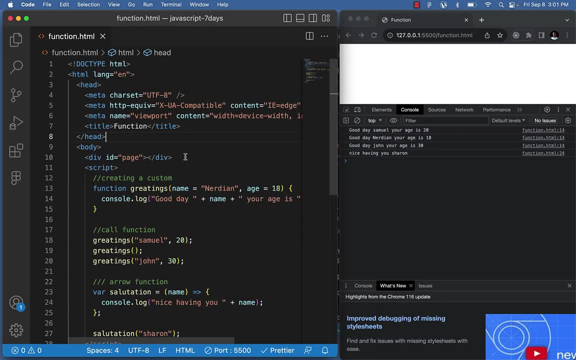 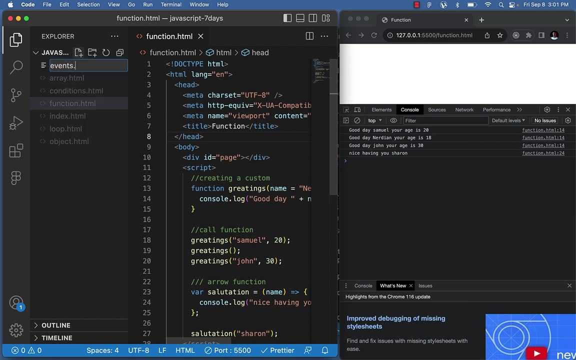 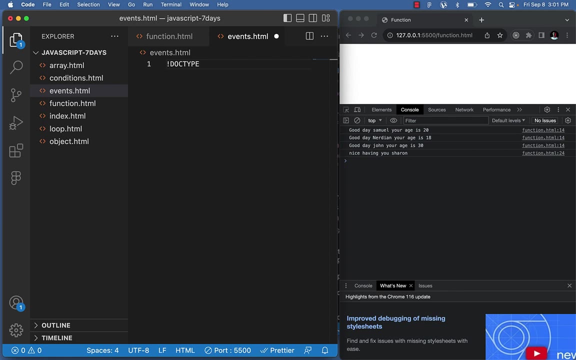 we're taking a look at door manipulation, event handling and door manipulation Basically, so I'll click here. I'll create a new file. Let us call it events, So we always do this for every video's HTML. Our basic structure, our basic structure, as usual. Let's just call it events and dom Close this other one. 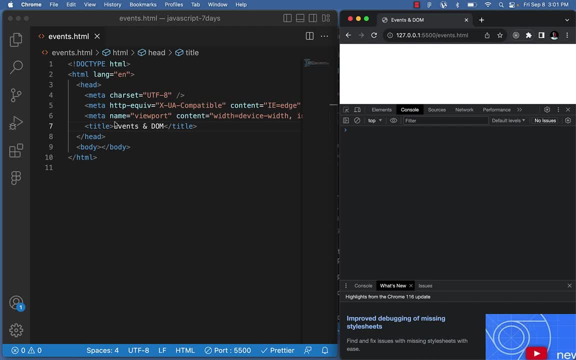 Let's run it here, All right? so now that we have it here, let's start again. So what exactly is a dom in JavaScript and what exactly is events in JavaScript, right? So I will start by explaining what a dom is, Then I will now explain what an event is, And I will now show us. 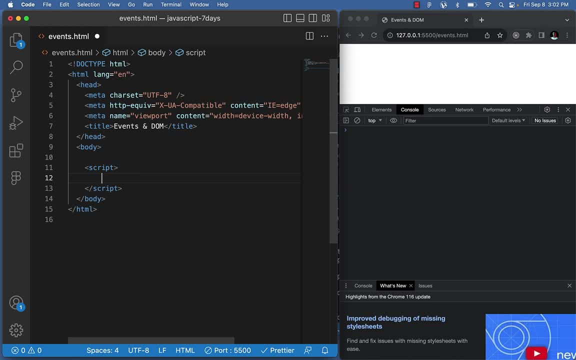 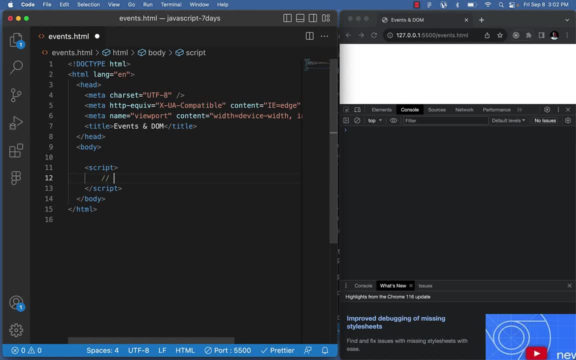 the first things want to talk about forces, you don't. so what exactly they don't? D dumb is like. this is how it's built: D o M right. so D stands for words, documents, all stands for objects and stands for model. alright, so this simply means that everything that we are 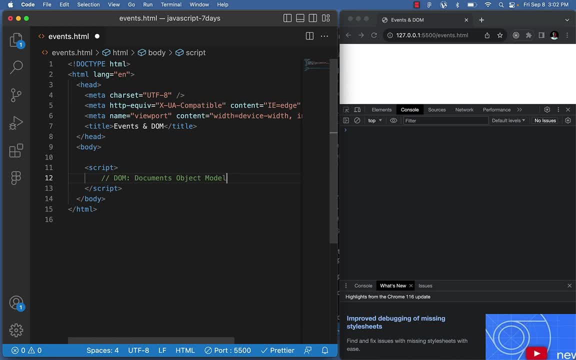 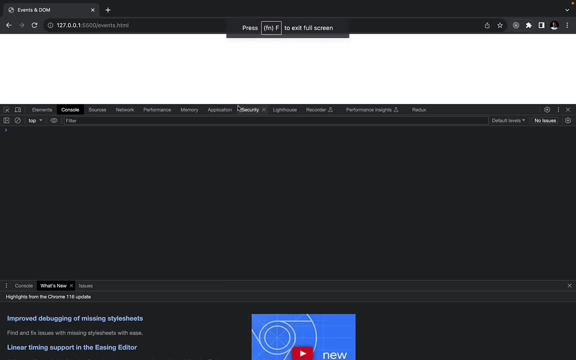 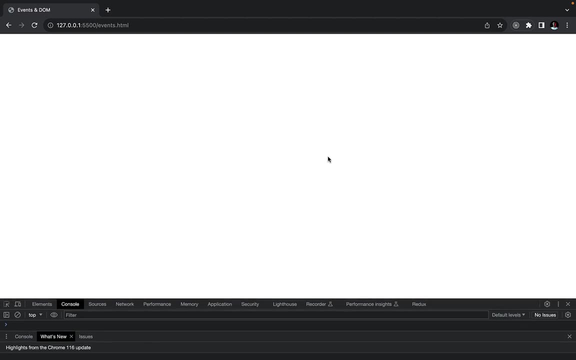 working on on cálculate that let me maximize this. this clarify, call. events and everything that you can see right here on this screen right now is our document, every single thing that you can see, this whole event, patient mail, is our document. so the web page on its own, on it's full, is 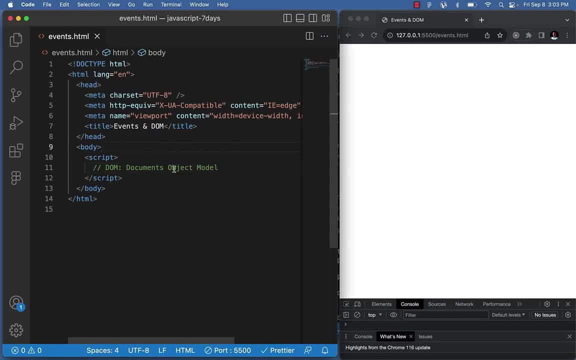 what our documents? right then. what then is an object? soup and objects reach out to you. right click on your product literally says perfect, this thing would be put into object. so basically, what one we have? our code here is an element. so each element, for example, this title like this, is an object. this meta tag is an. 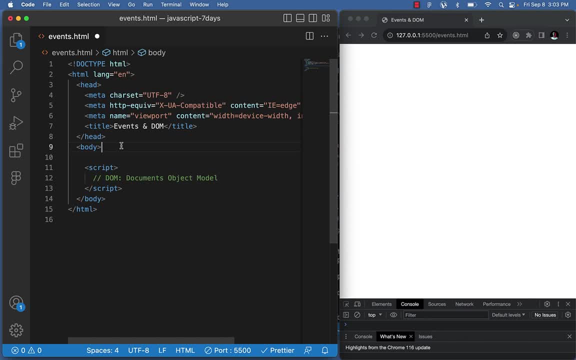 object. this head as a whole is an object, then the model is basically the arrangement, the fact that we have title instead of head, and we have head and body instead of the html. so everything put together makes up our DOM. so everything that you can see like this makes up our DOM. so, if right, 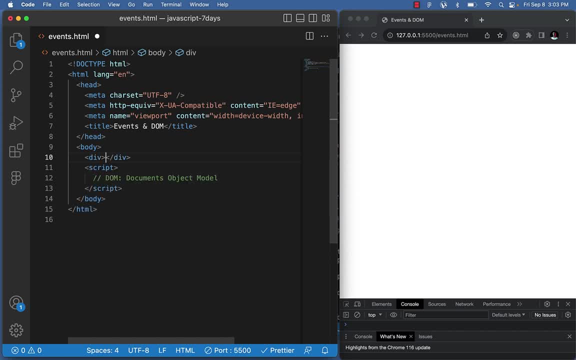 here we have a div, a html div, that says: this is this is a, this is an element, this is an element, right? so instead of our DOM, we have a div that says this is an element. now let's say we have another thing. again, we have a button, and in this button we just want to put change me, for example. 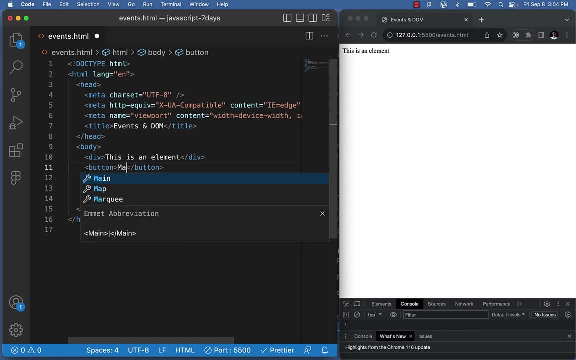 uh, manipulate DOM. let's just manipulate DOM, manipulate DOM. so when, when you hear the word DOM manipulation, so event handling and DOM manipulation, so the manipulation comes in when we want to programmatically change the content of our DOM. in other words, we want to programmatically change the content inside our web page. so by so doing, we 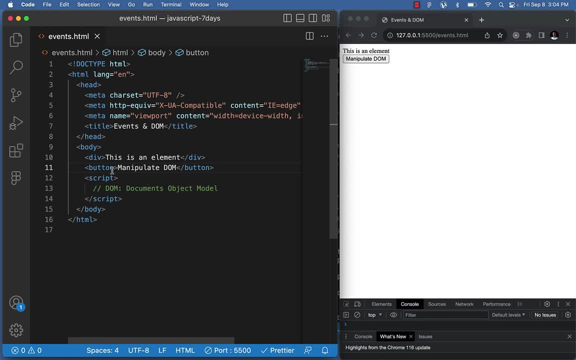 are manipulating our DOM, right. so let's say: if someone click on this button, we want to change this. this is an element to the DOM have been manipulated, right, so that is how we're going to programmatically change it. so let's programmatically change it without um using any form of event, so we can now. 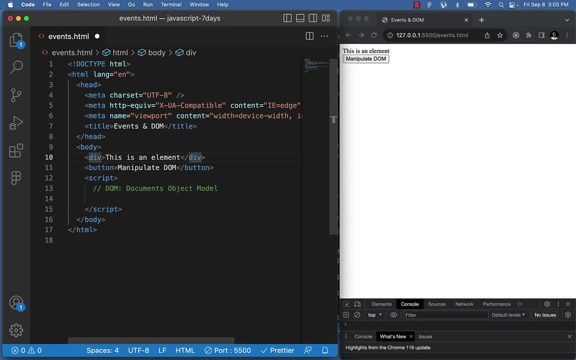 do something like we can now get the value of our DOM. let's say: this has an id. id is equal to. let us call it um el. let's say short word for element: right, so now for us to get that particular id so we can manipulate our DOM. we get to use a selector so we can manipulate our DOM. we get to use a selector. 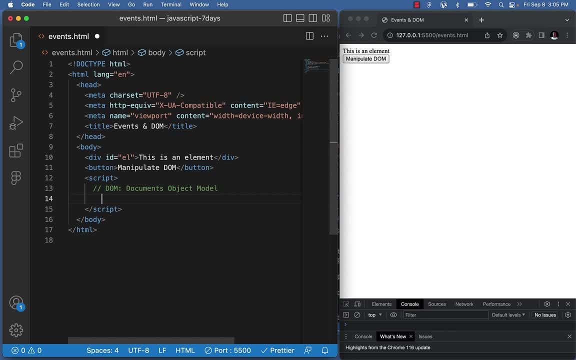 in javascript, which is an inbuilt function called um, um documents dot. get elements by id. this element is capital letter e, the b is capital letter b, the iso capital letter i. so this is an inbuilt function or method instead of javascript. right, and it carries an argument. that is the id. 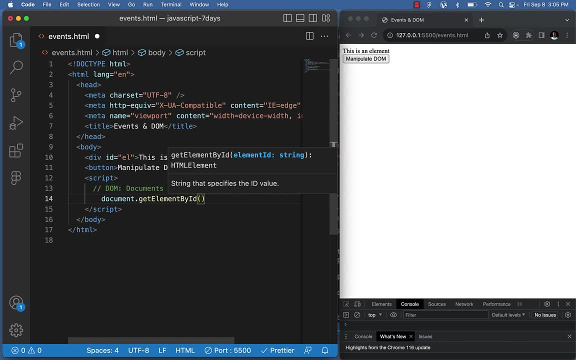 of the element that we want to select. so in this case, the id of the element is el. now we also have another um inbuilt element in javascript in this function that is called inner html. so inner html allow us to manipulate our DOM by imputing a new content into our DOM. 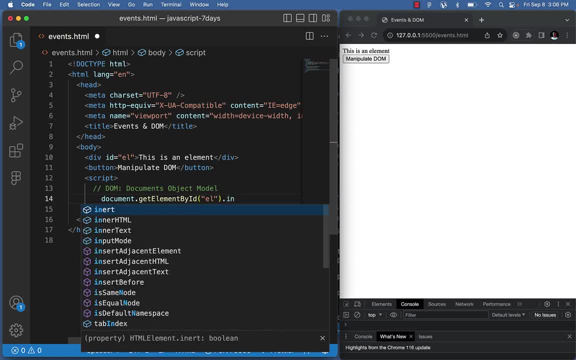 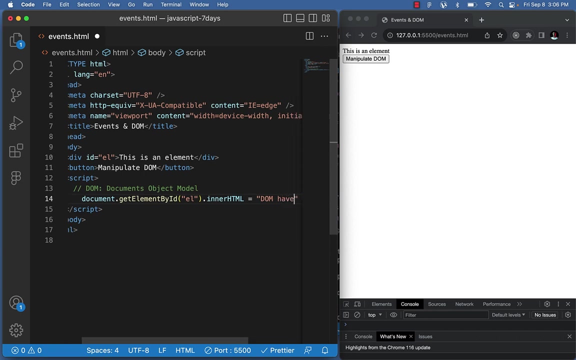 so we'll do that by saying dot- inner html equal to. so this equal to will carry the value that we want to impute into our DOM. so in this case, the value i want to put into our DOM now is viva domain. it is viva domain. 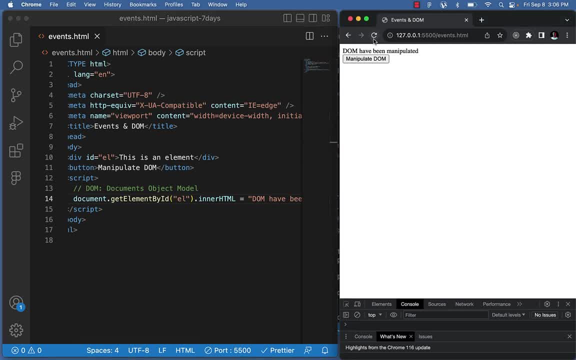 of the menu um have been manipulated. let's just use the word dom. Using JavaScript from this element, that is, the original content to DOM- has been manipulated. That means we have done what DOM manipulation- So changing the content on our web page- is called DOM manipulation. 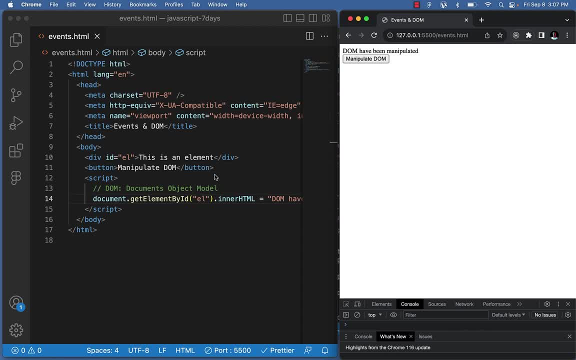 Now, what about event handling? Now, for us to understand event handling, we need to first and foremost, know what exactly is an event. What do we call an event? So an event in JavaScript or in web development generally, is every interaction of the user. 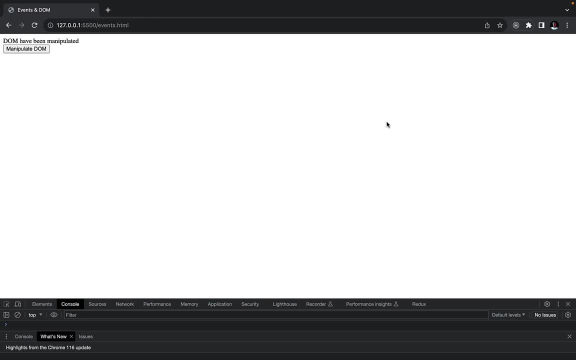 For example, the way I'm moving my mouse here. this is an event actually, right, So I'm moving my mouse. I'm putting my mouse on top of this particular button. It's called the hover event. If I scroll, this page can be scrollable. 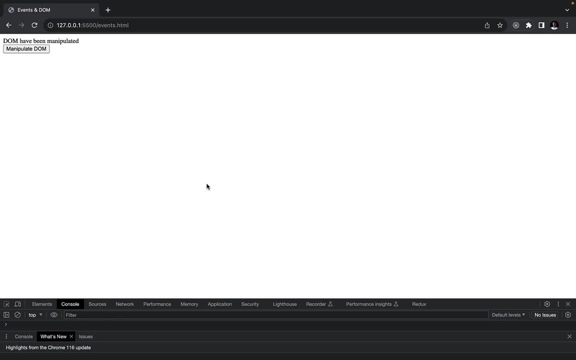 It can be called on scroll event, right, So we have different kinds of events. So, if right here now, If right here now, I want to click on it, So we have the on click event. So we have several events. 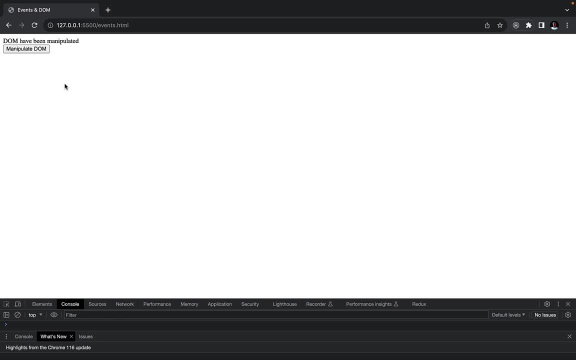 On click event: when something is being clicked On mouse over, when we have your mouse over an event On scroll, when you're scrolling through the web page- So many kinds of events that we could have. So let me minimize this and create an on click event. 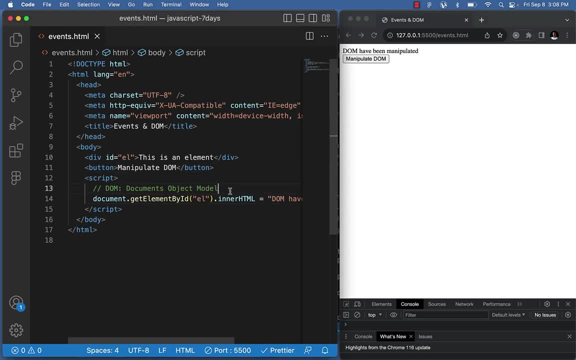 For an on click event. what we are going to do is we are going to, first and foremost, create a function, So let's call that function. change DOM or manipulate DOM, So let's call it, Let's say function. We are going to say function. 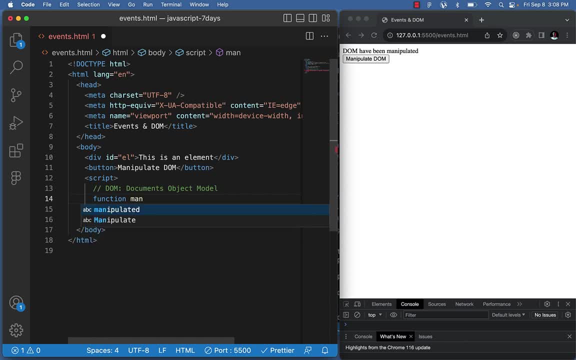 It'll say short form: manipulates DOM, Something like this. So we are going to have something like this. So if this function is being triggered, Right, So these are elements- If this function is being triggered, this DOM is going to be manipulated. 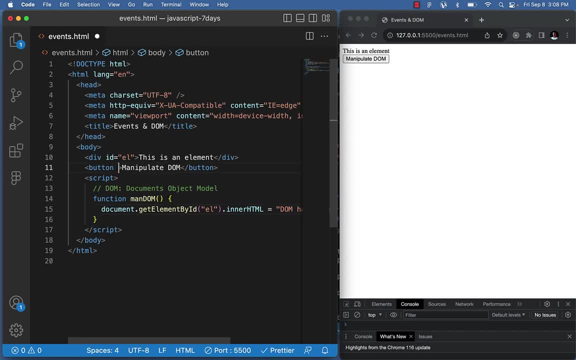 And we're going to have DOM have been manipulated. So for us to do that, we'll come over here. I will say on click, Which is the event that we want to get now. So we'll come over here and we'll say: 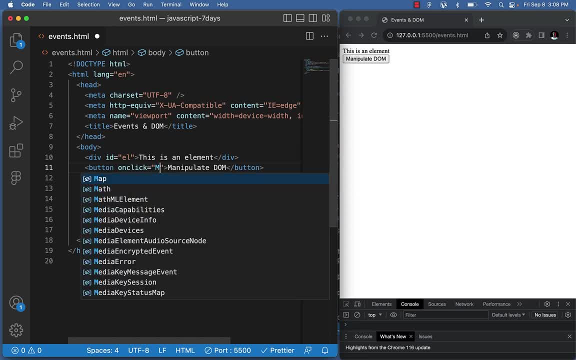 When they click this. what we want to do, We want to call this function, call- Sorry, MN DOM, manipulation, So something like this. So this is the function I want to call when this particular event is being what, When this particular button is being clicked. 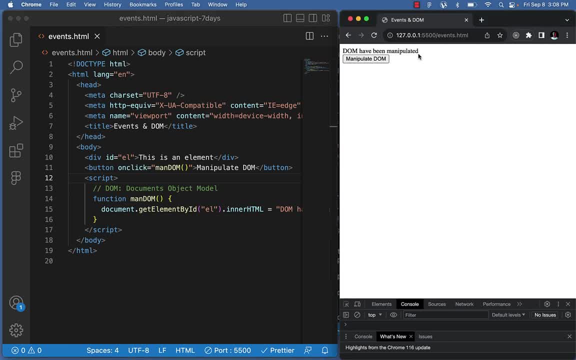 Let's click it now. You see, DOM have been manipulated. Let's refresh, Click it again. DOM have been manipulated. So with this, now We've handled the event on that particular button. And the event that we've handled on that particular button is called what? 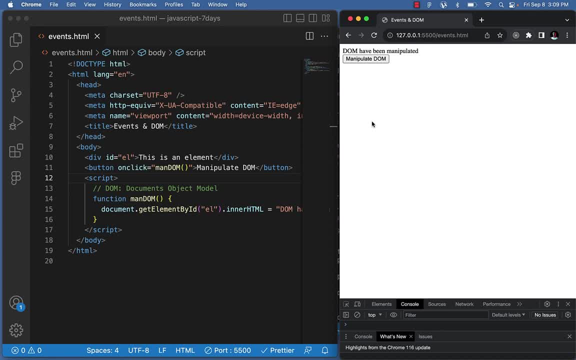 The on click event Right. So now, If you dive in deep to learn more about DOM manipulation and event handling, You're going to see several other ways that you can actually select an element. For example, You can get document. Get element by class name. 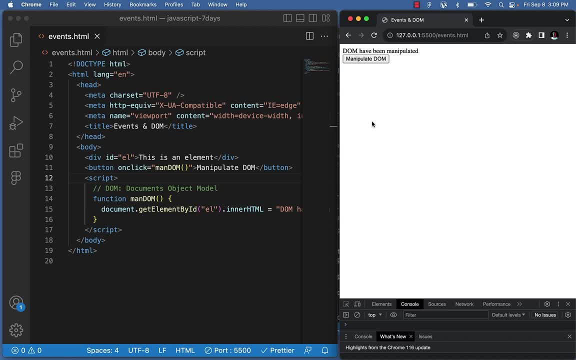 We have document by query selector. There's another one too, as well, That you can use to get your element. You can also get your element by tag name too, as well, So you can now quickly do a Google search And you'll be able to see several ways you can select elements. 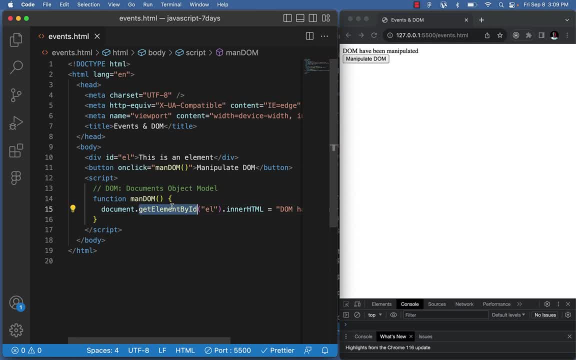 Apart from the document, Document, Get element by ID, As well as other events, too, that you could also get. Now, one other event That would actually love us to also try and see Is the event on form handling, For example. 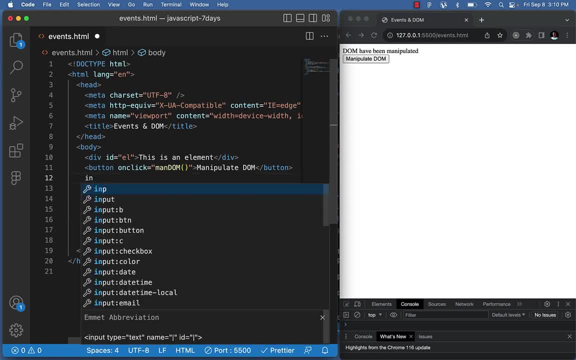 If someone types something in an input field, Let's say: this is an input field. now, Right, Someone will be able to type, Let us say: Let's give it an ID. Let's say ID, Let's call it input, For example: 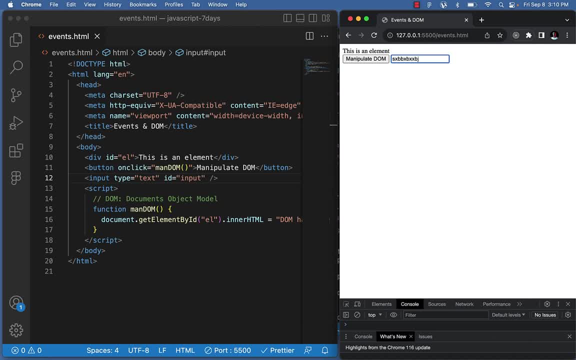 So this is an input text And I want them to be able to type something here. And on type, Let's create another button. Let's say this button now is called what- Submit. So let's say the value of this button now is called submit. 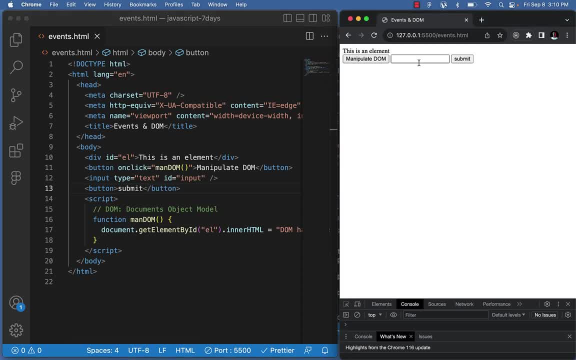 Right, Aha, So one such a way that once you type something here, You click on submit, Let's alert it, So I will be able to see it. So for us to do that, Let's create a function. 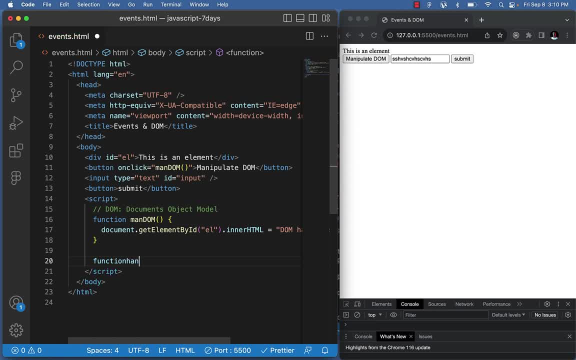 Right, And let's call this particular function handled form. Oops, I did not give space here Handled form. So if we have handled form Like this, Right And aha, So we can now get the value of our form. 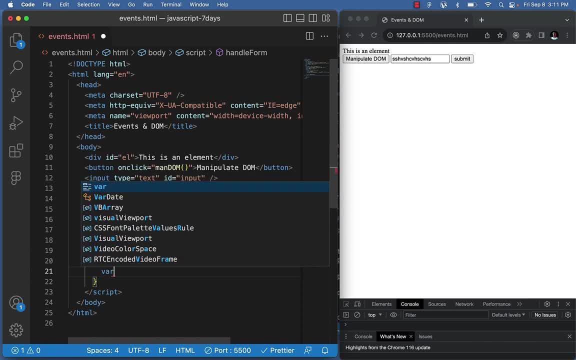 So we can now say: Let's say, for example, Variable Text Is equal to the value of this particular form. So the value of this particular form, The value of this particular form, will be Documents. That gets elements by ID. 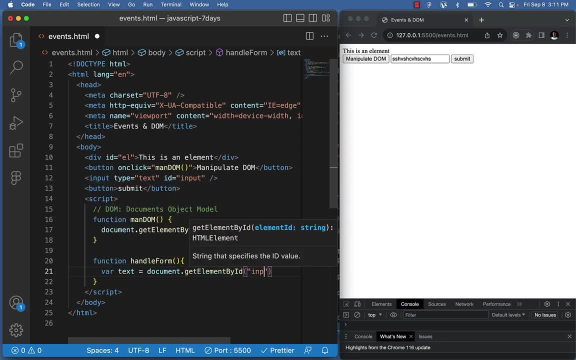 The ID now will be Input. Remember, That's how we give it Dot value. Right, Input dot what Value? So all we just need to do now Is to say alert, Or we can use console log, But let us use alert. 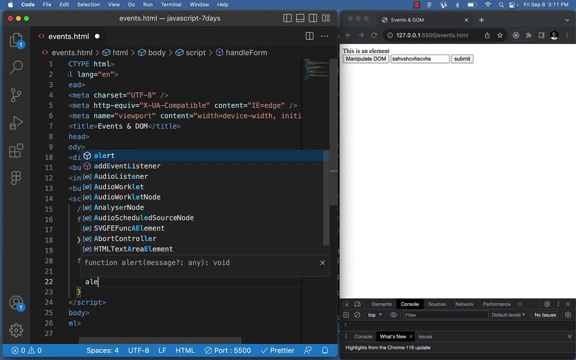 Alert input dot value. So right here now We will come over here to the button Where we have on click, We say on click, We are going to say On click, We are going to say On click, On click. 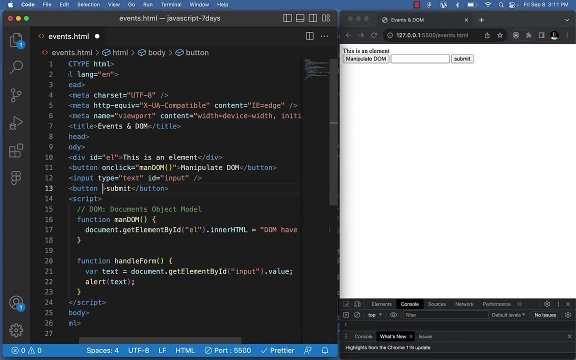 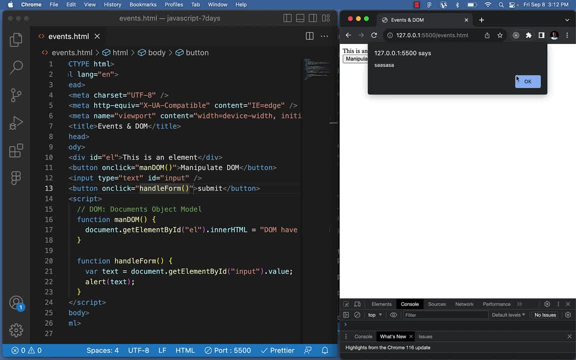 If I type something here, I am expecting to see What I typed here, Something I typed. Let me type. something Makes more sense. Let me type Um, Um, Um. Serving these JavaScript. Alright, Serving these JavaScript. 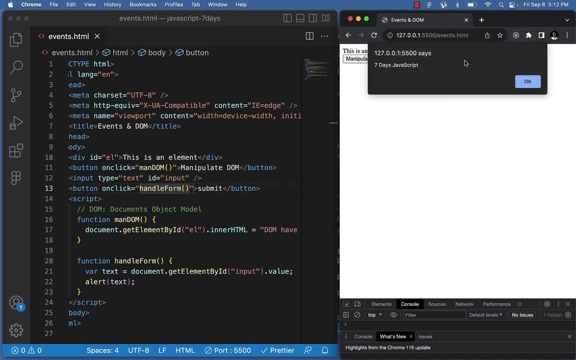 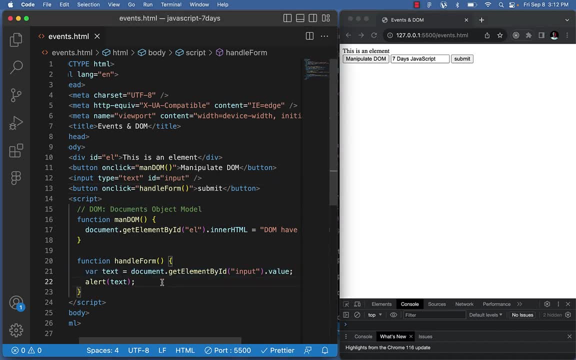 Some. it is Serving these JavaScript, Right, we should. so anything I type here, If I click it, it's going to alert it for me, right? So that is us learning door manipulation and event handling. now, mind you, There are different kind of events handling. you could check that out with Google search to learn more on these things. 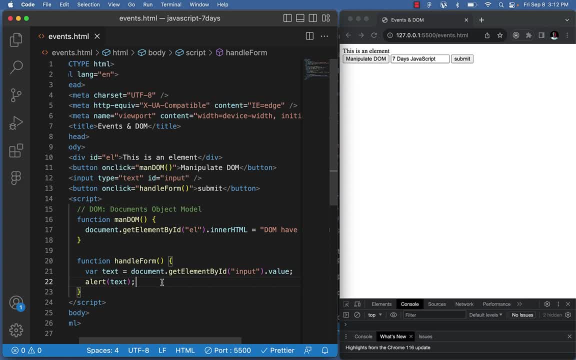 So you can learn a little bit more deep. It's just like the unscroll, The unscroll, unhover, unkeyup, unpressdown. These are several events that you could actually handle, but this is just basically What you need to understand when it comes to door manipulation and event handling. 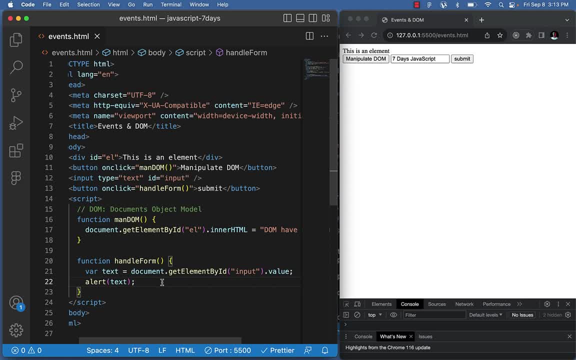 So thank you guys for watching this particular video And thank you guys for joining us in this seven days class, and I hope that we all enjoyed it. Peace out. 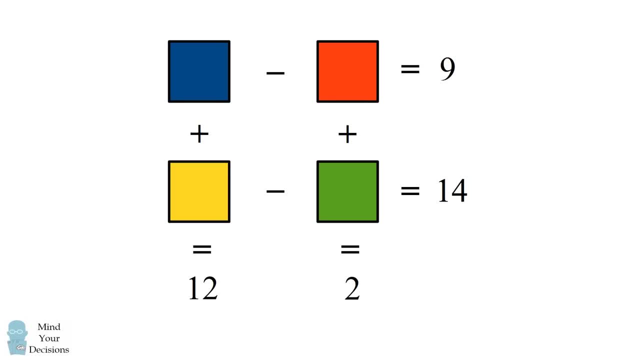 Hi, this is Presh Talwalkar. Can you figure out this problem which is driving people crazy? Your job is to put numbers in each of the four boxes to make all of the equations true. Give it a try and, when you're ready, keep watching the video for the solution.